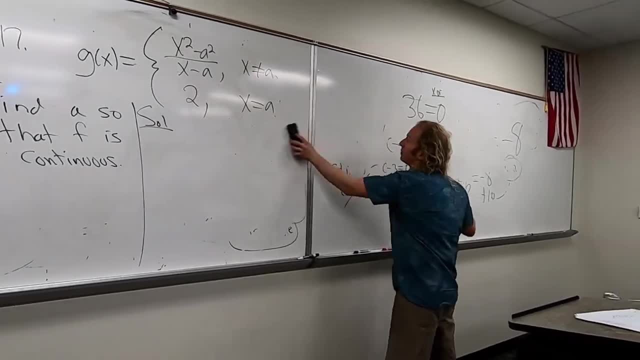 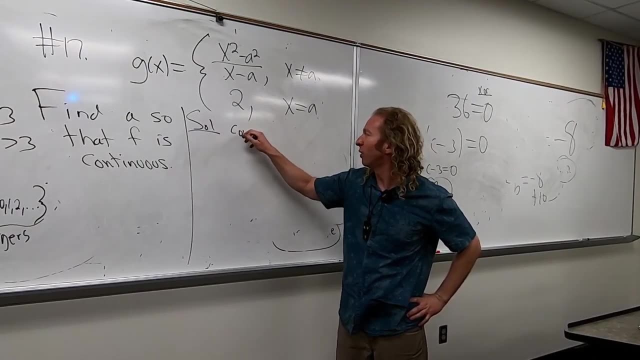 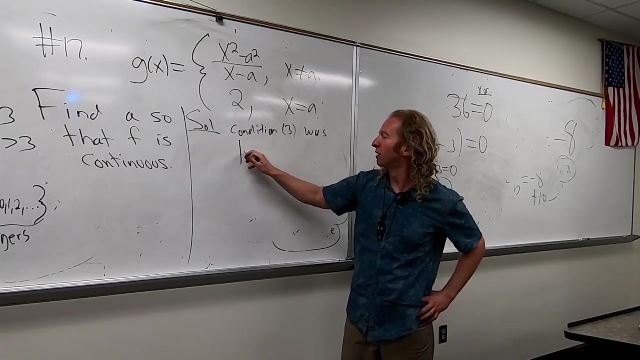 Well, what we have to do is use the third condition of continuity. The third condition of continuity so was that? condition 3, I'll write it here- was limit as X approaches A right. That's what we care about here. A of G of X. 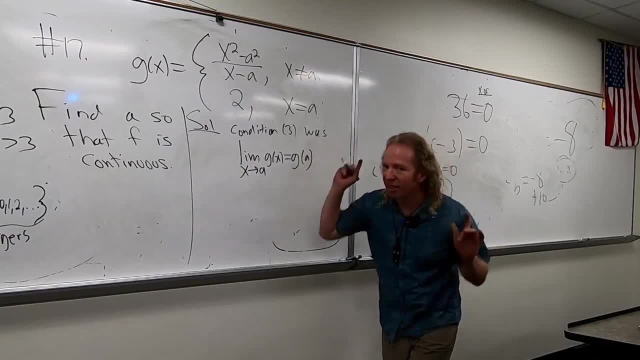 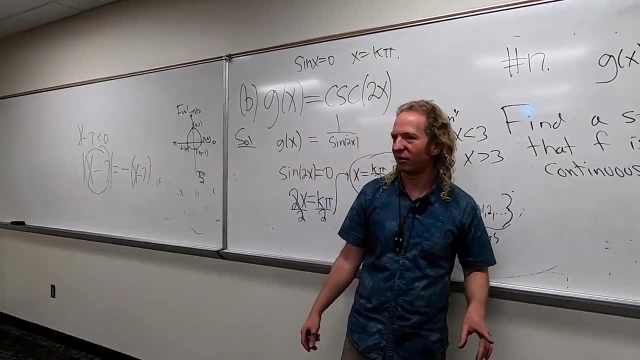 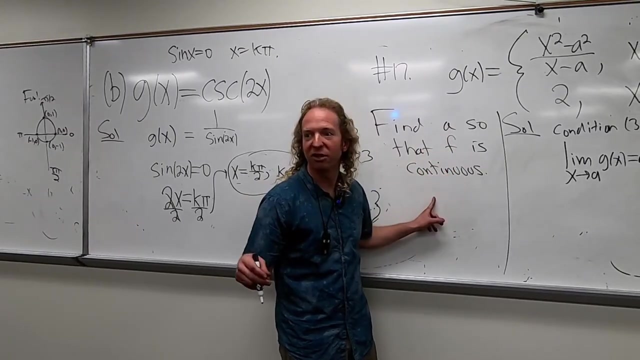 equals D, G of A. That was condition 3.. I just replaced G with F and C with A. I think I said that right. Yes, So wait, you said: find A, Find A, so that F is continuous. Wait, is it? F is continuous. 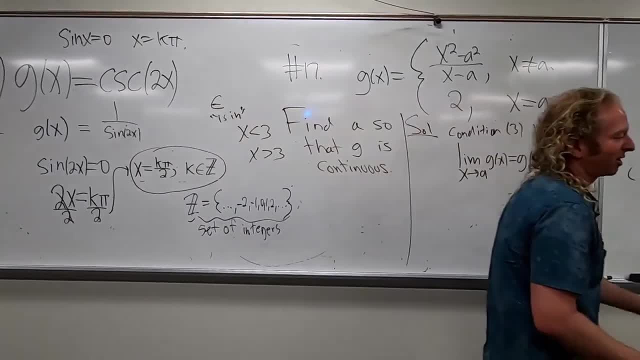 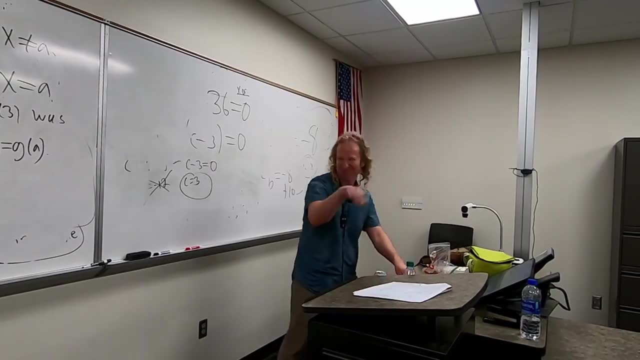 That's supposed to be G, Okay, Okay, I should just give you all the points. Okay, Logan. and what's your name? John, John, That's good, that's good, That's all right. It doesn't affect my life, right? No one sees your grades, it doesn't matter. 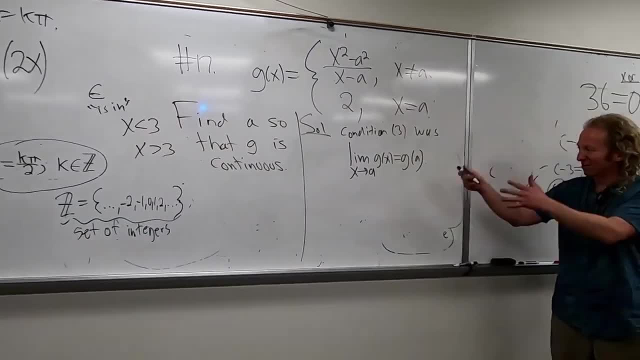 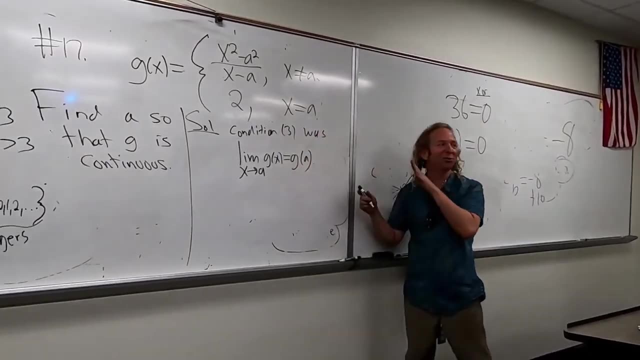 Okay. so condition 3 was: was: that doesn't? doesn't? it has no effect on my life? Yeah, it doesn't matter. In 20 years it won't matter, Okay, so we have to do this. So so that's condition 3.. 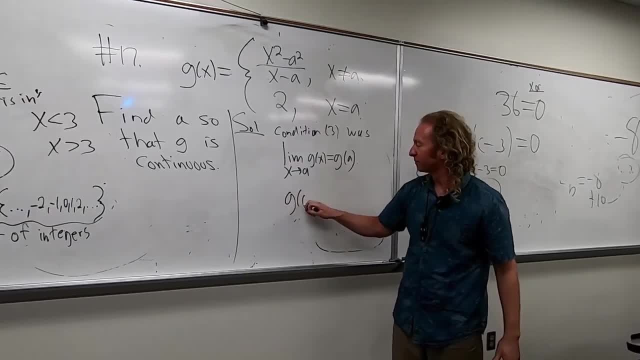 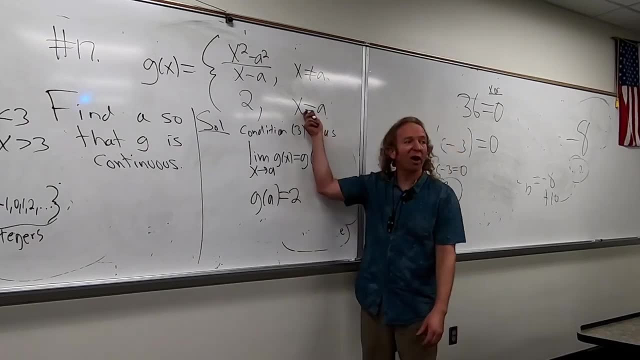 So let's go ahead and work out this piece. first, G of A. So G of A is equal to what would G of A be in this case, 2.. Very good, Logan, Everyone see why it's 2?? Because when X is A, you get 2.. 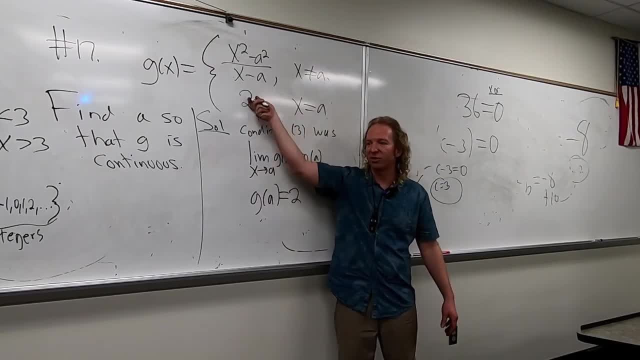 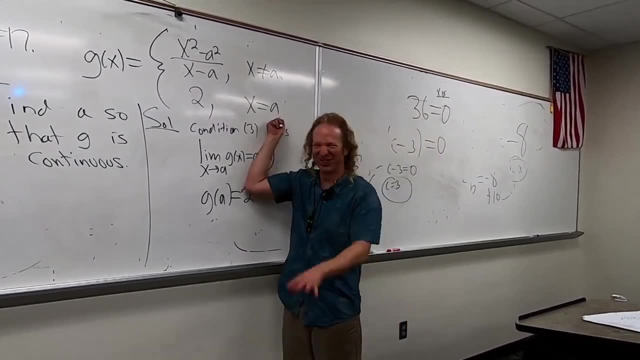 Right, when X is A, you get 2.. So G of A is 2, right, G of A is 2.. Bless you. I saw it coming. I saw you, like, start to sneeze. I'm like, oh, she's going to sneeze. this is too sorry. 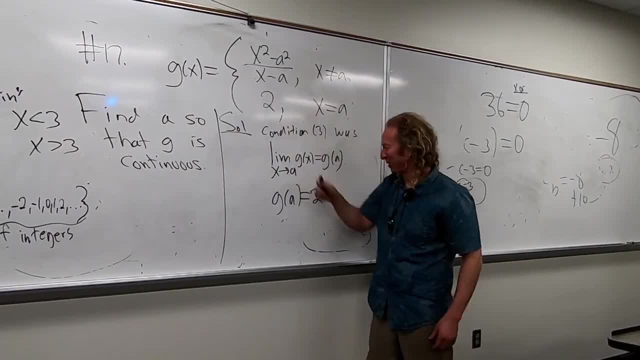 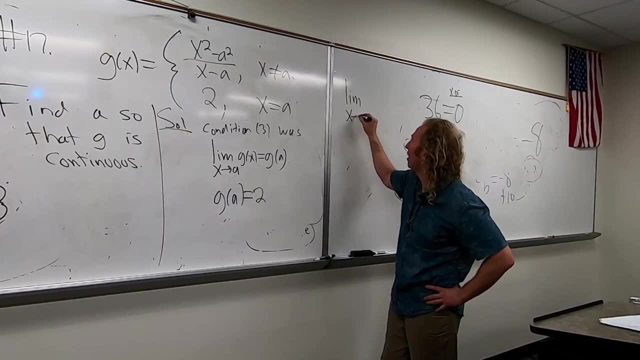 So G of A is equal to 2.. G of A is equal to 2.. All right, so now we have to use this condition here, So I'm going to go ahead and write this down: Limit. this is where I was like what's going on? 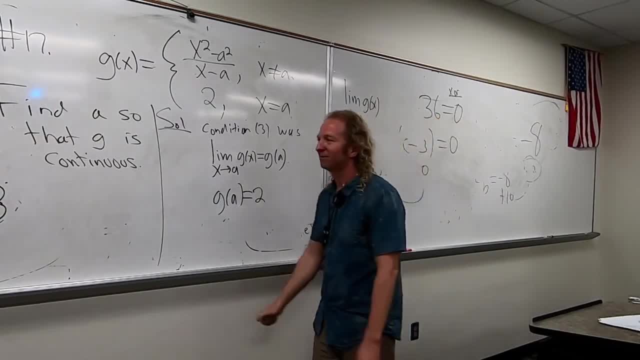 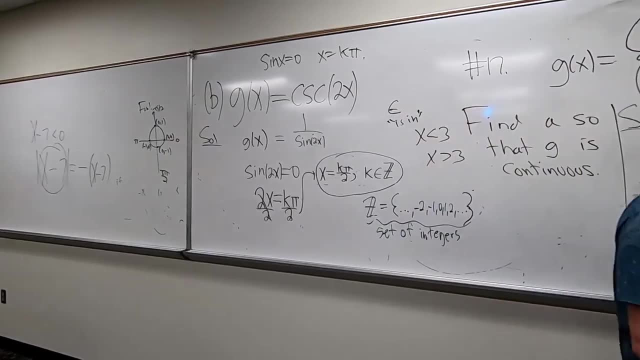 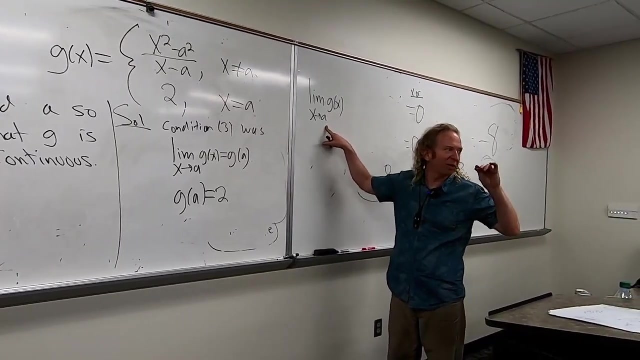 Like: so I? I think I said this the first day of class, But I never wrote it down. So when you're taking a limit, you only care about what's happening when X is close to A right. You don't care about what's happening when X is equal to A. 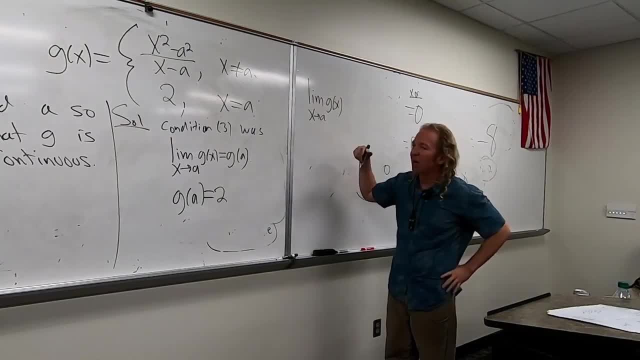 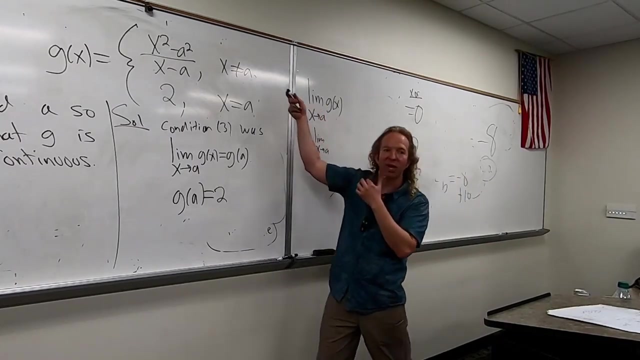 So, in fact, during during this entire process, in your mind X is not equal to A. So, because you only care about what's happening when you're close to A, so X is not necessarily equal to A. So in this case, when X is not equal to A, we use the tuple.